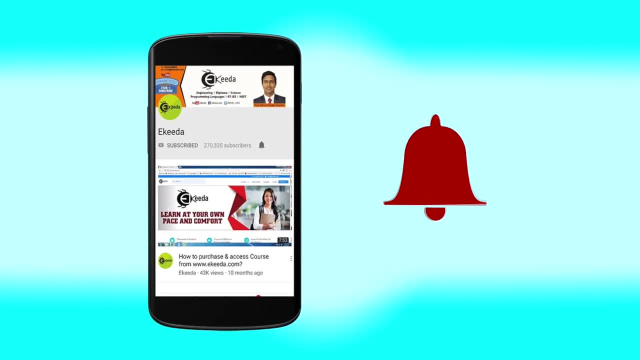 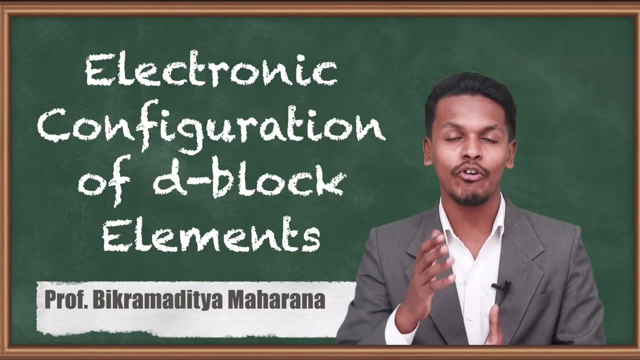 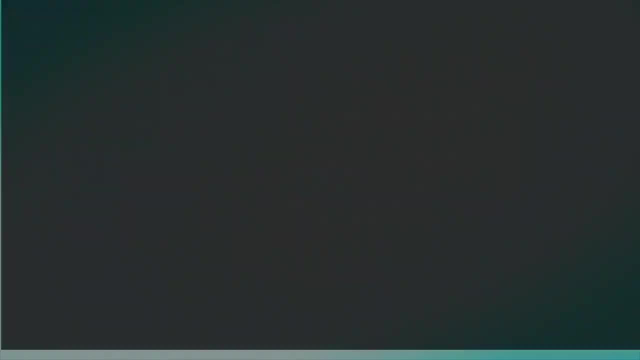 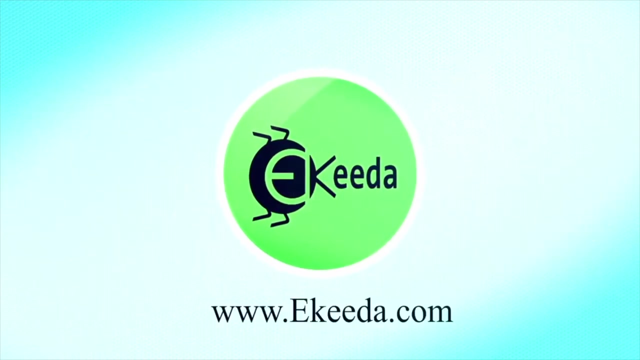 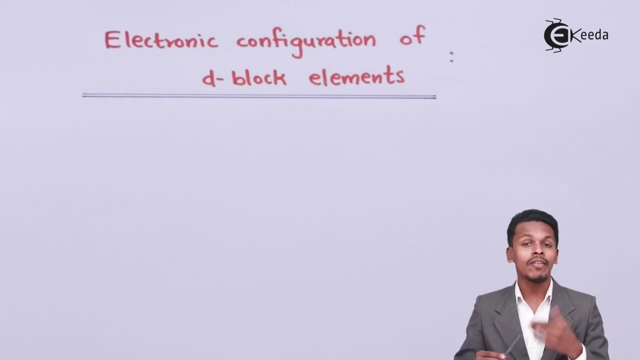 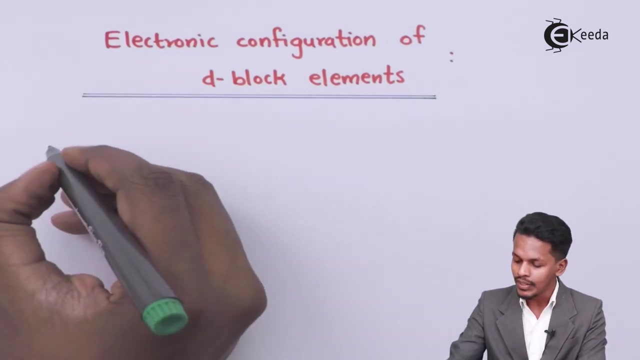 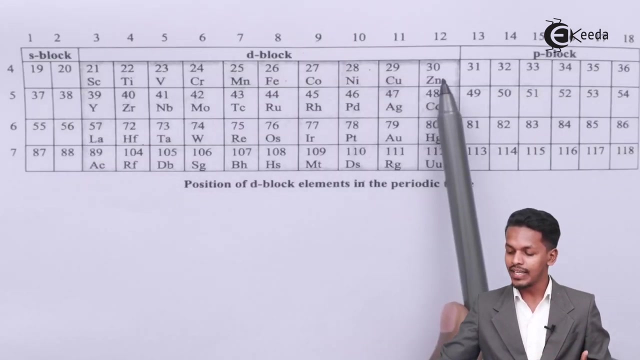 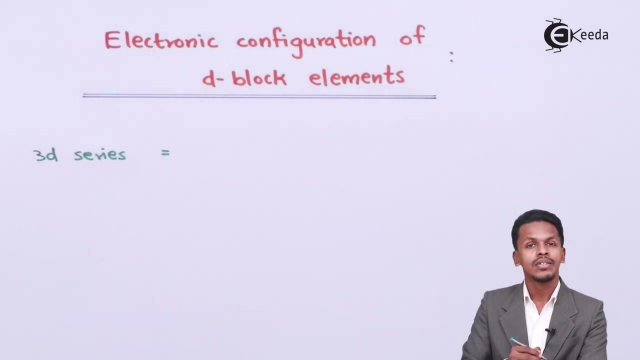 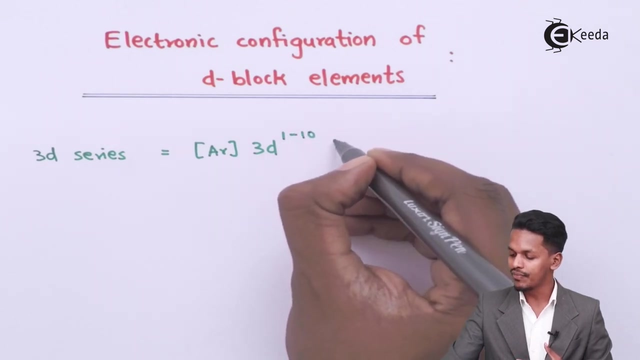 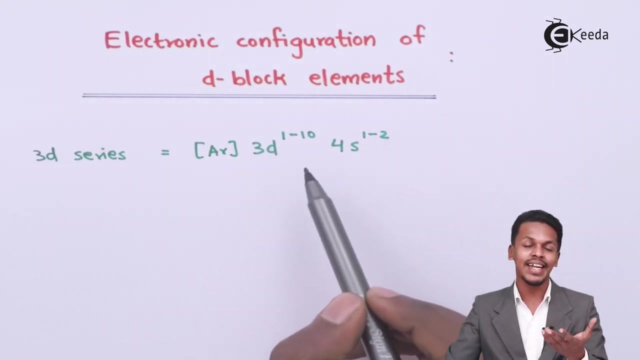 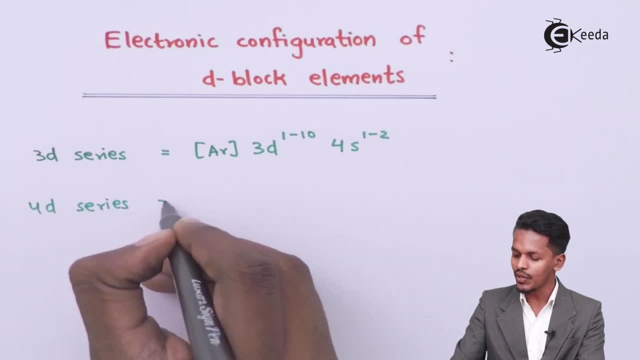 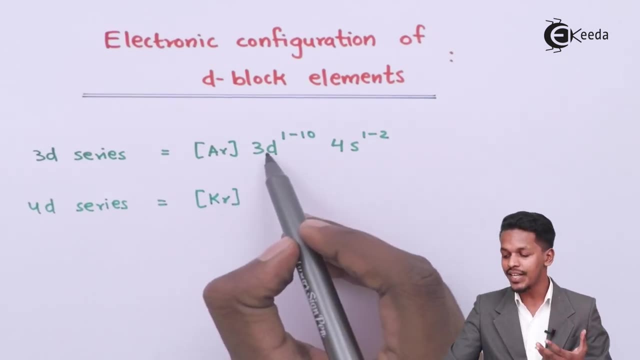 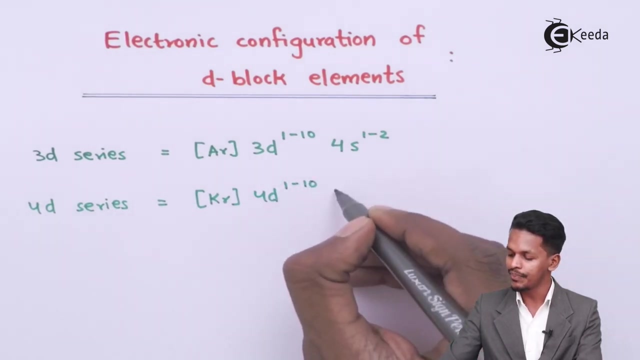 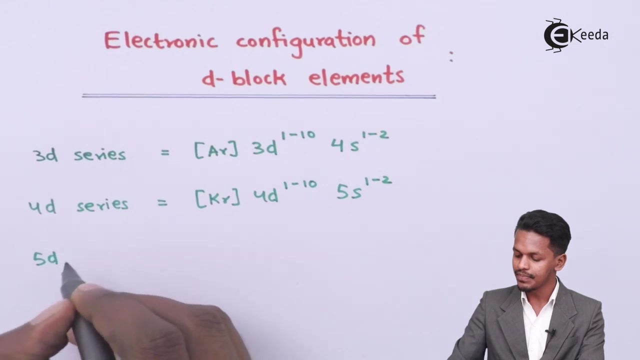 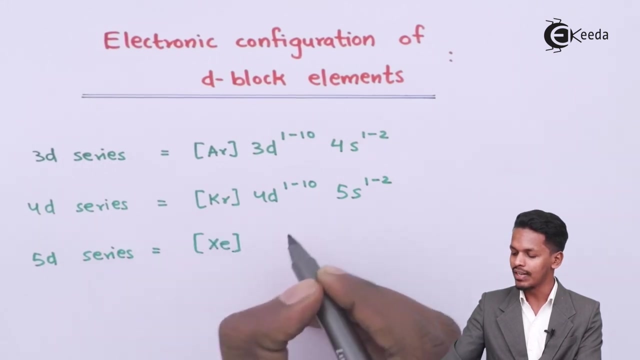 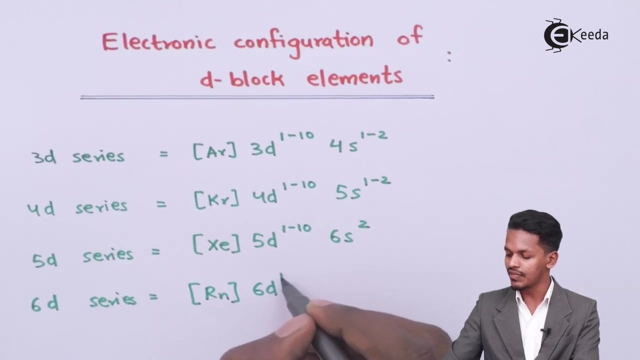 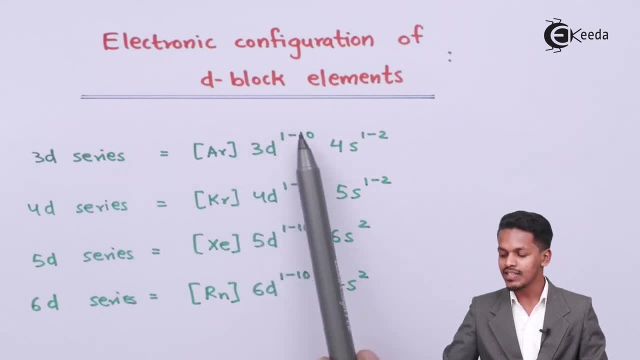 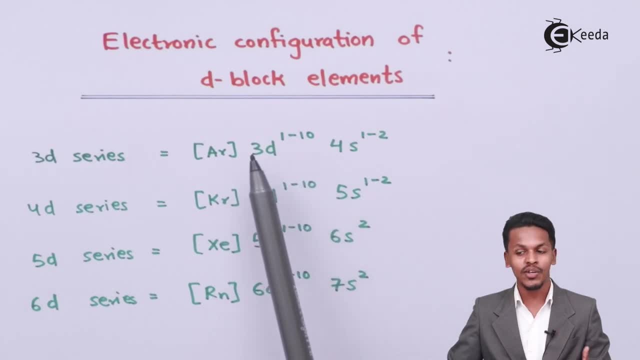 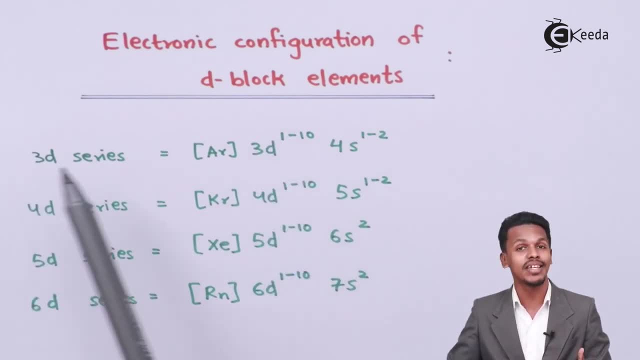 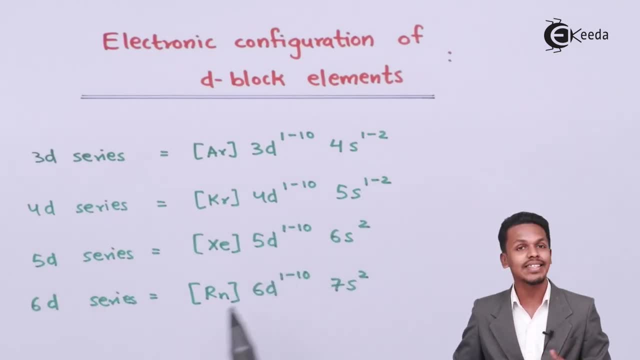 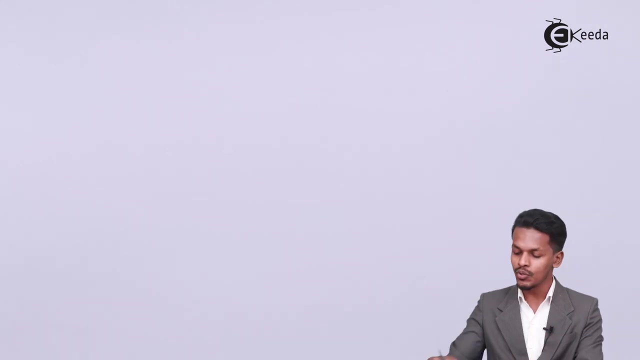 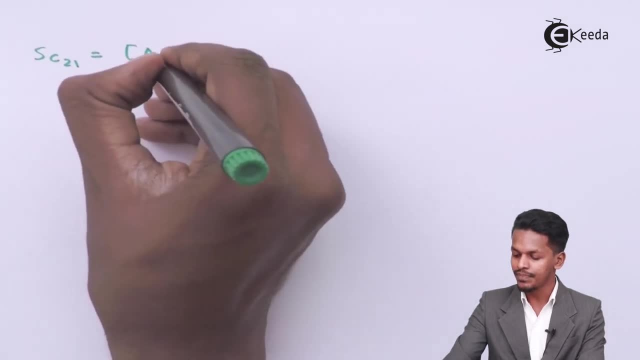 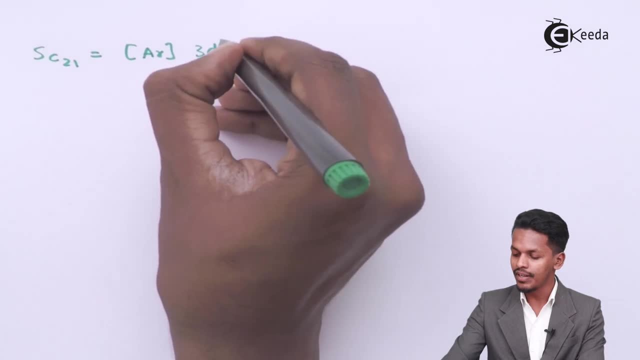 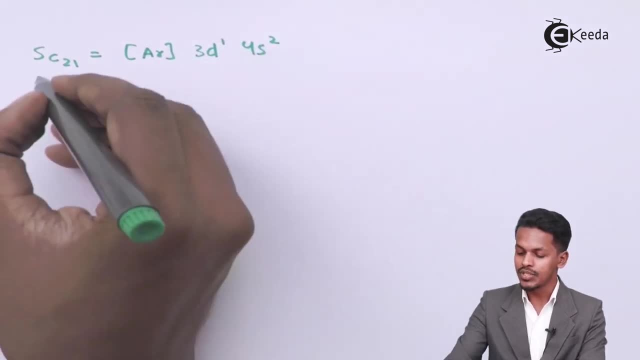 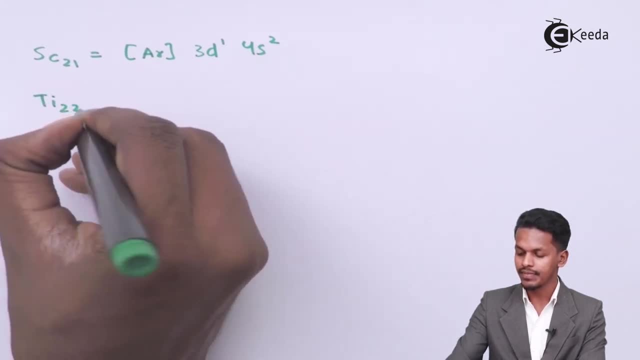 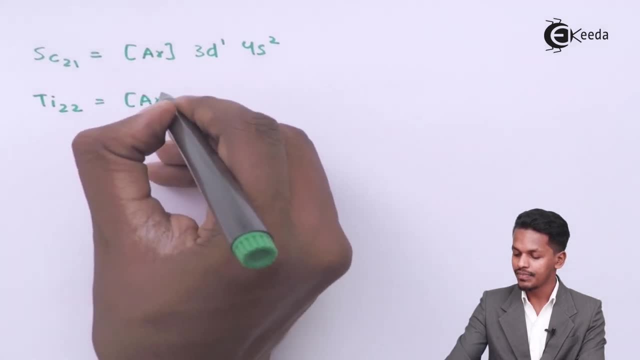 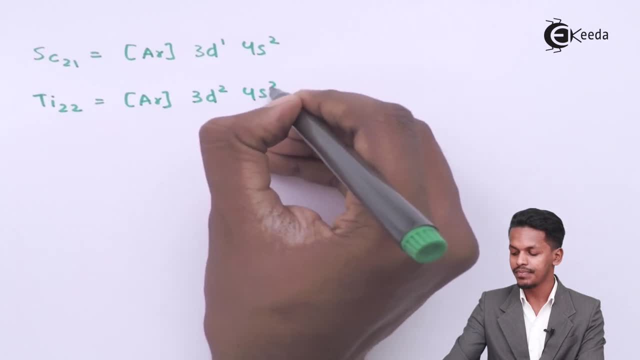 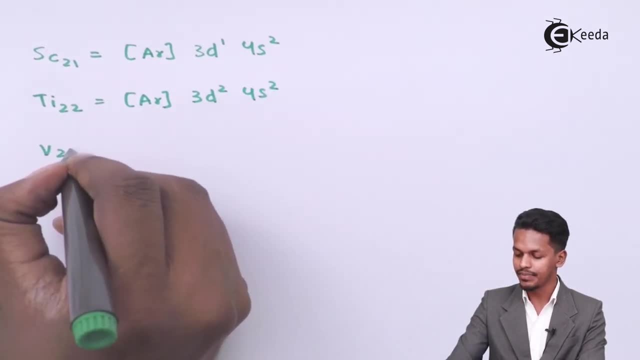 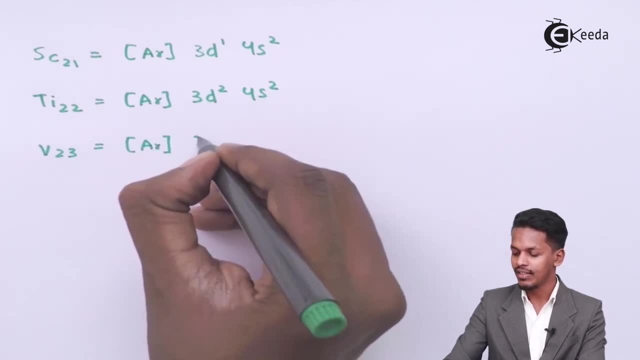 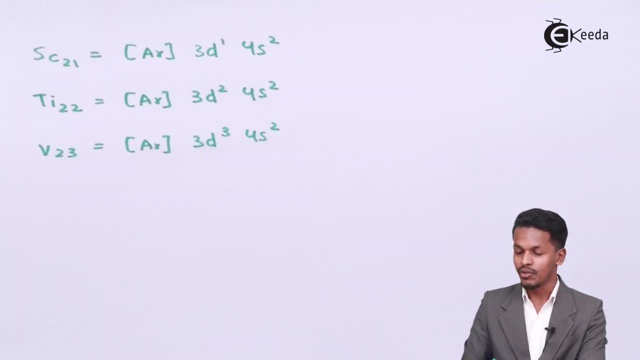 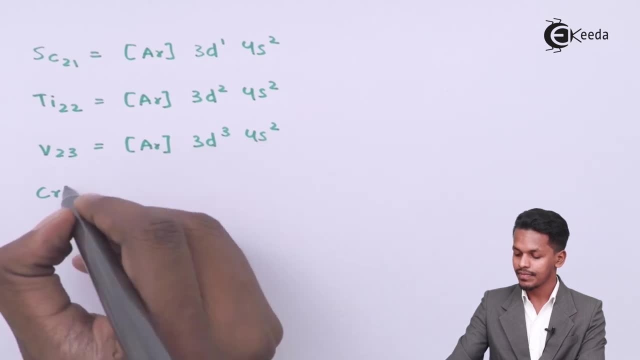 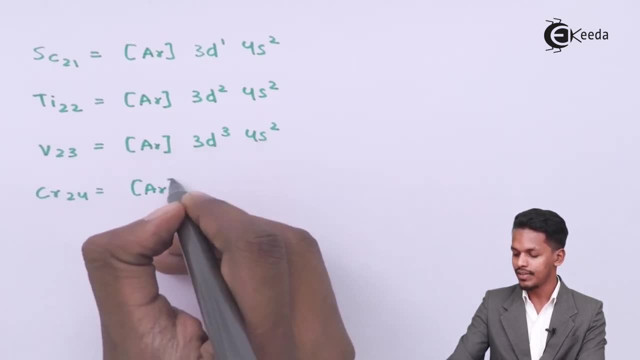 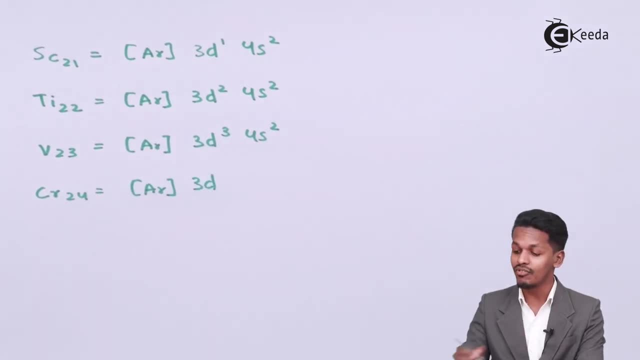 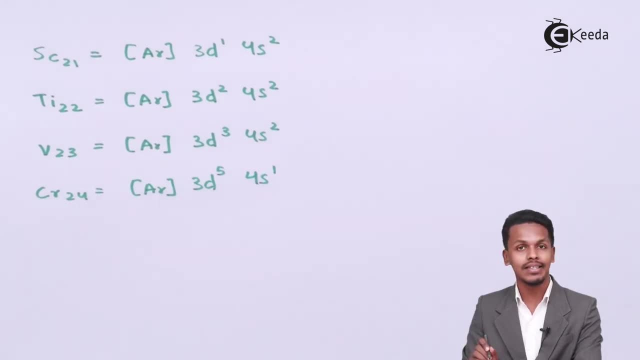 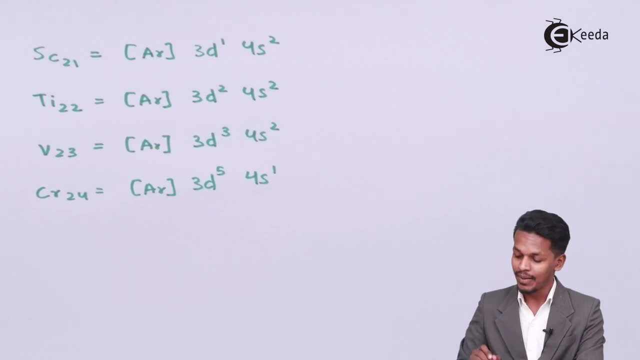 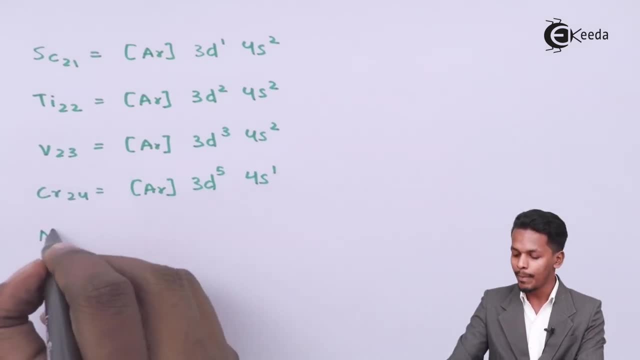 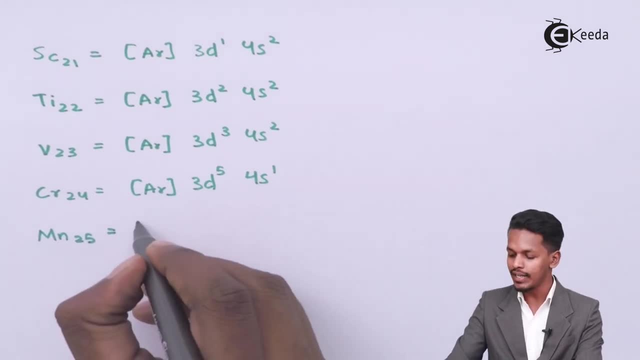 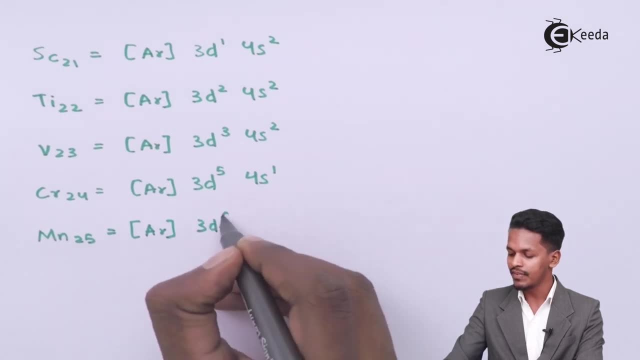 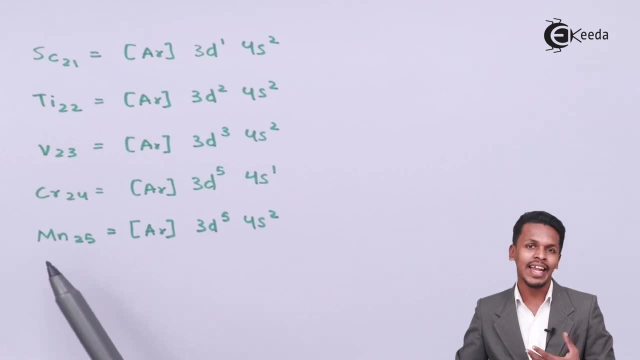 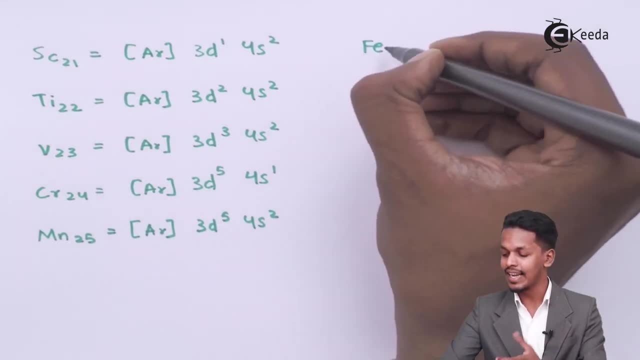 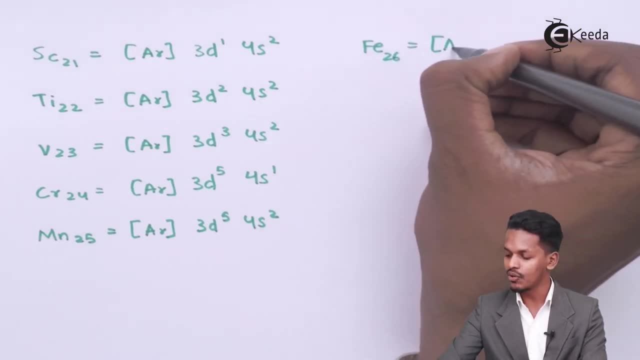 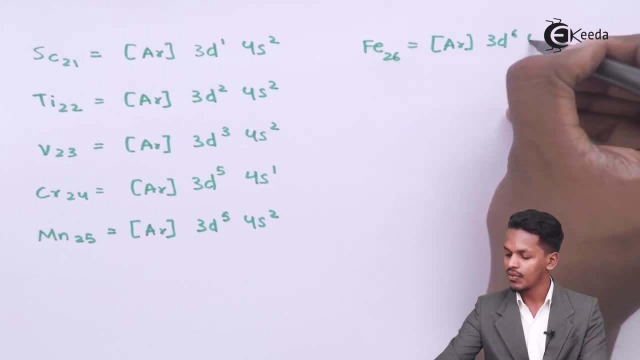 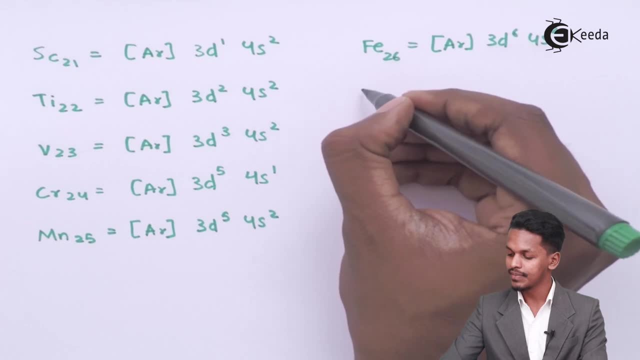 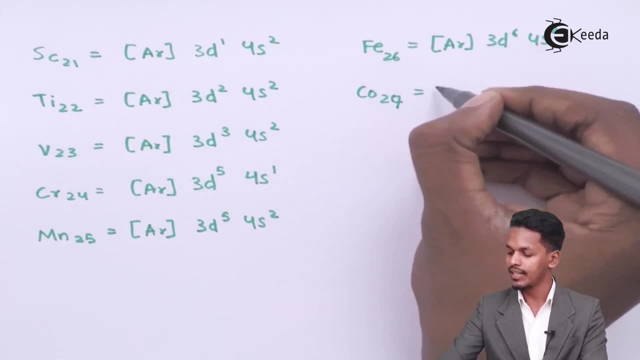 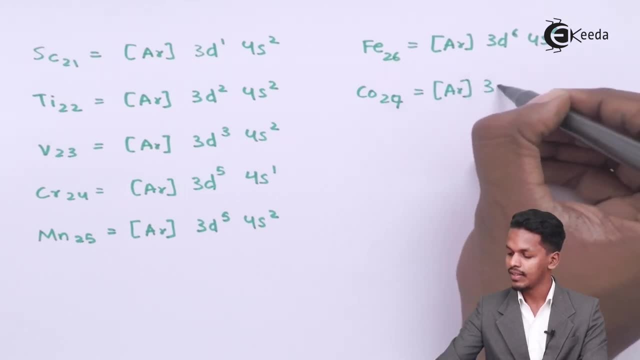 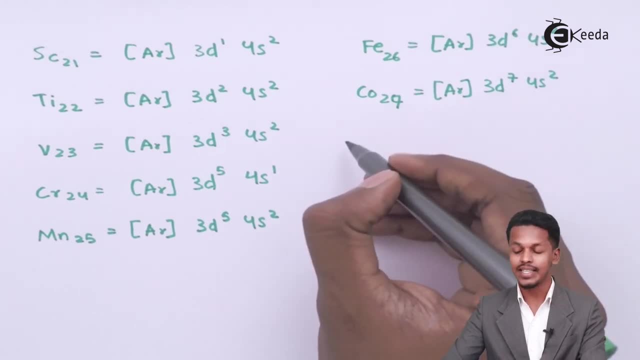 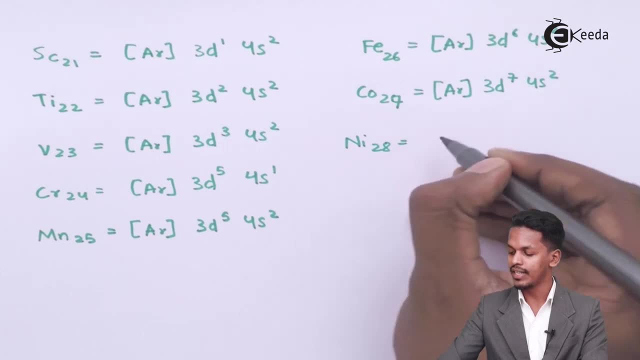 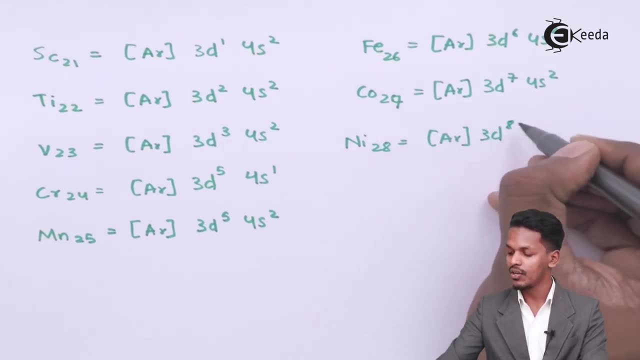 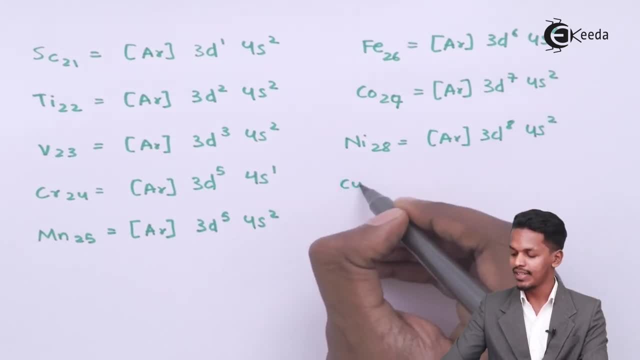 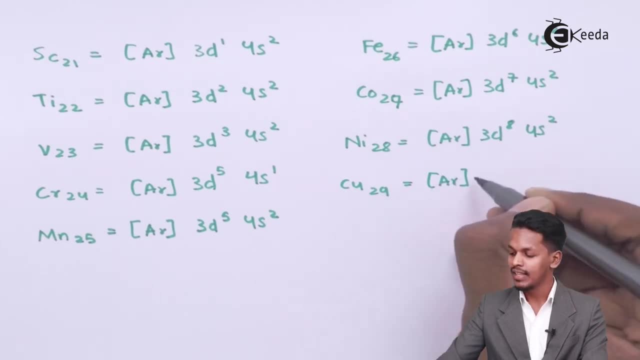 Click the bell icon to get latest videos from eKIDA. Click the bell icon to get latest videos from eKIDA. Click the bell icon to get latest videos from eKIDA. 3d10, 4s1- even. i am going to talk about this one, i talk about the next one. that is the last one.